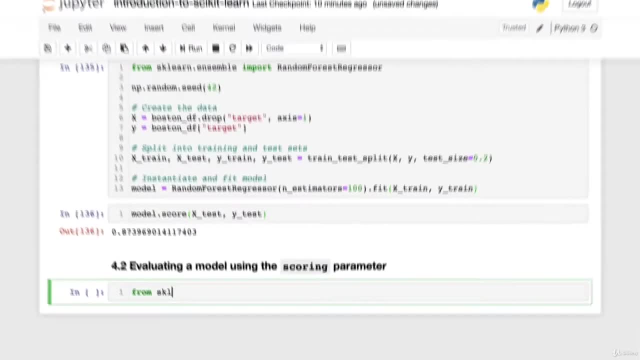 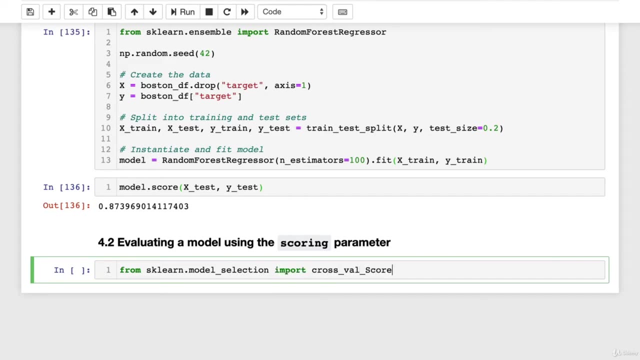 So let's get started. What we're going to do is go from sklearnmodelselection import cross-val score And, as always, we're going to run it. So we're going to run the code first before we dive into what's actually going on. 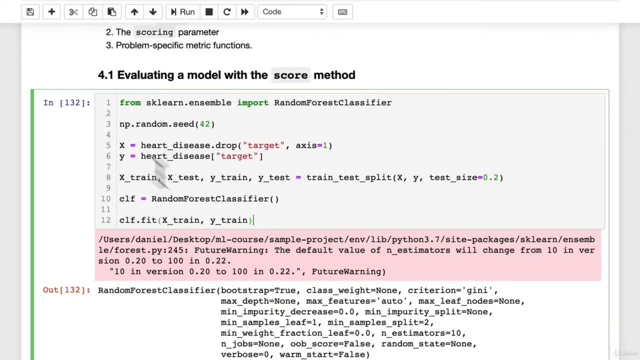 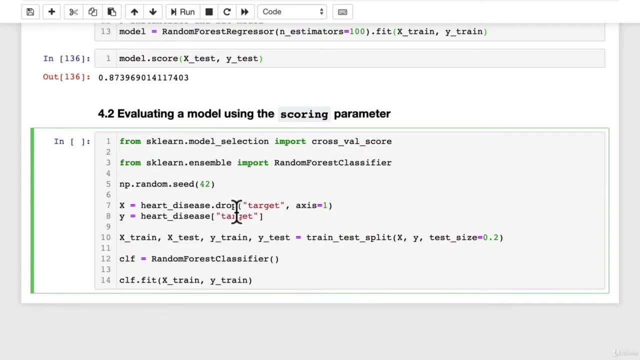 And what we do need is some classification code. So what we're going to do, we can copy this. You're allowed to copy this, by the way, because we've written it a fair few times now. So only thing different here of what we've done is we've imported cross-val score from scikit-learn's model selection. 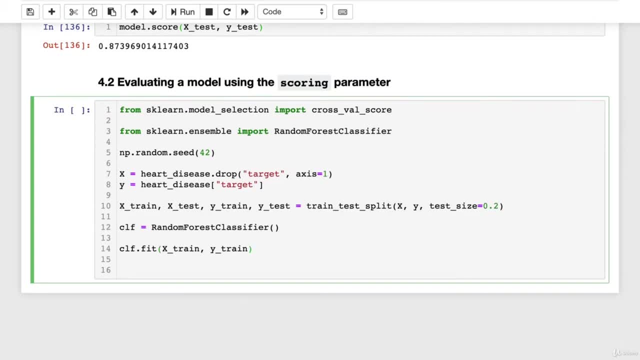 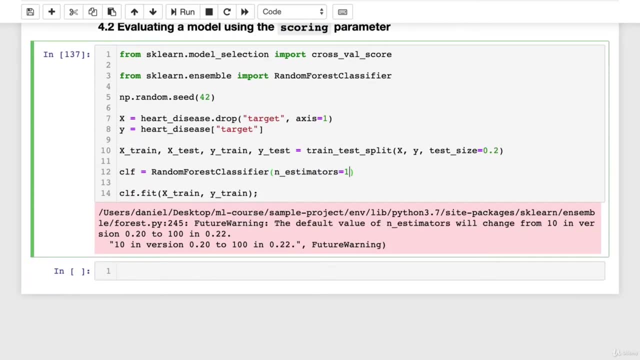 Now the next thing we're going to do, because we've called fit there, we'll just put a little semicolon so we don't get a big output. You know what? this warning keeps coming up, so we might just keep changing that to: nestimators equals 100.. 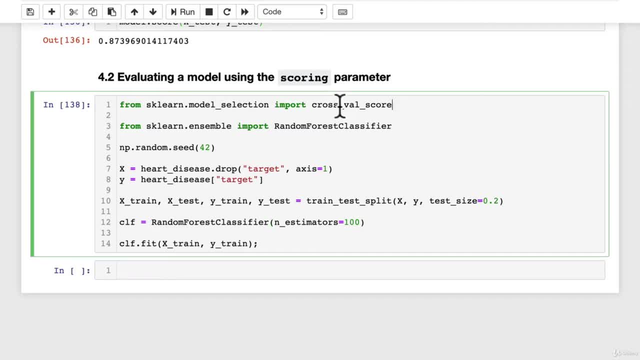 Wonderful, And so cross-val score. It has the word score in it, but we've seen what is this cross-val doing? Well, let's have a look. So go, cascore, we're going to do the test data first so we can compare, and then we'll do the same. 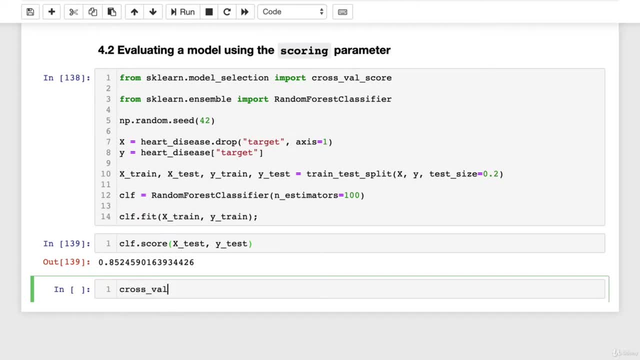 But this time using cross-val score. Cross-val score and cross-val score takes our classifier. it takes the x-data and it takes the y-data, Not the test and not the train. We'll see what's going on in a second. 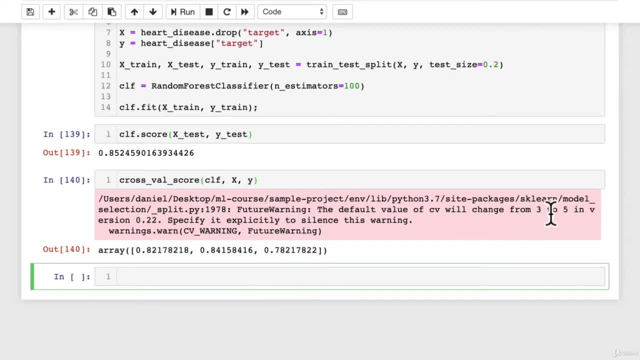 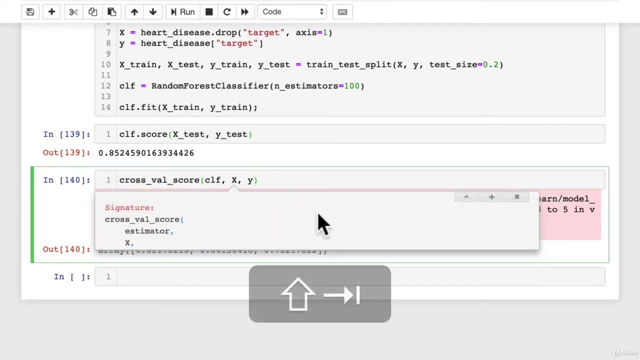 Ah, what's happening here, And again we're getting another warning. This is just to say that the default value of cv will change from three to five. So if we have a look at this shift tab, Let's read the doctrine. 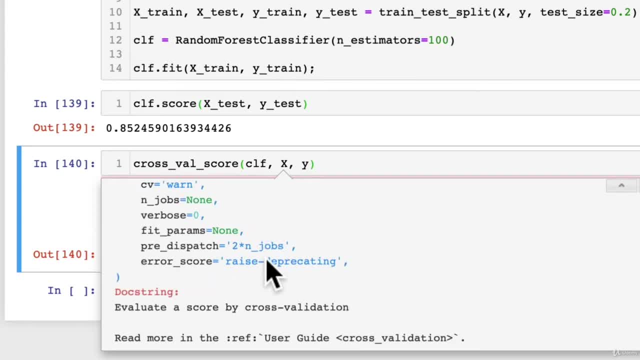 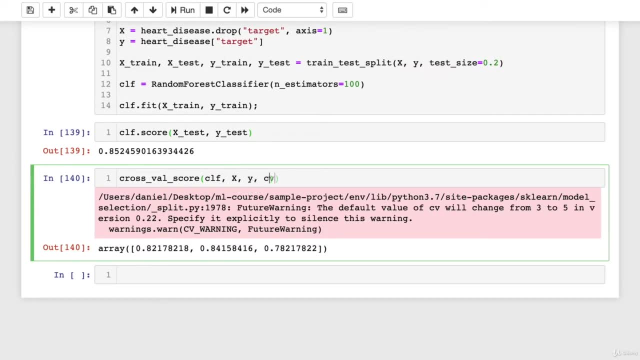 Evaluating a score by cross-validation. What even is cross-validation? And so cv is going to give us a warning. This is where that warning is coming from. If we change this from, cv equals, the default is three. if we change it to five, that warning is going to go away. 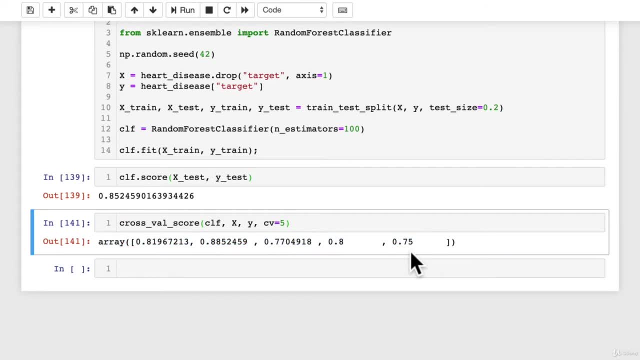 And then we're going to get an array back of five different scores. Hmm, So that's probably the first difference that you'll notice: Cross-val score returns an array, Whereas score Only returns a single number. Okay, so how can we figure this out? 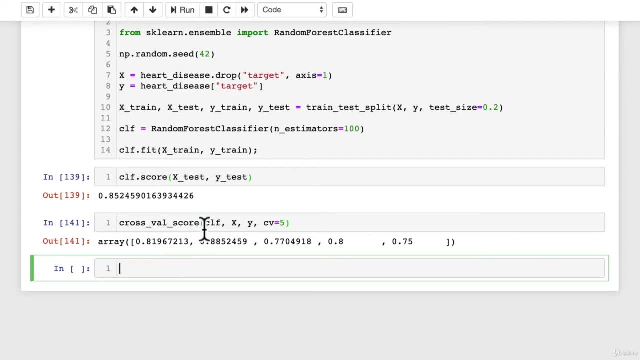 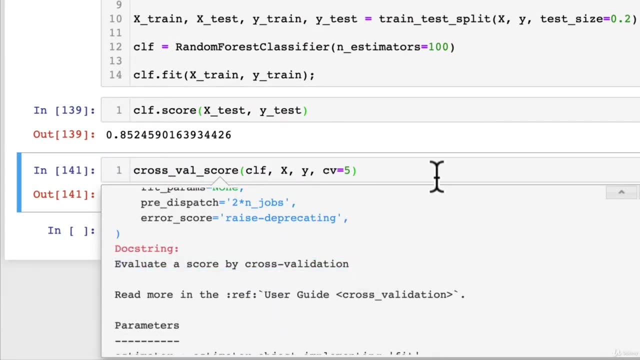 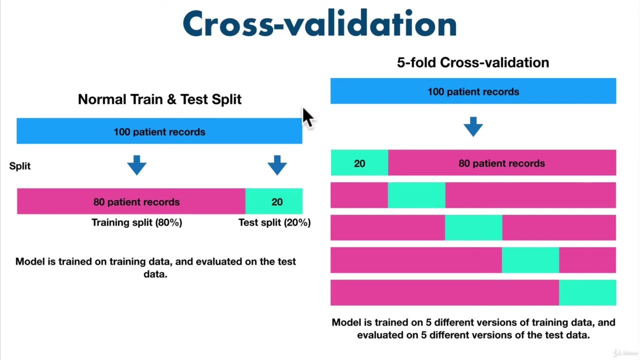 We need to figure out what cross-validation is, because that's, after all, what cross-val score is doing. Come back into the doctrine: Evaluate a score by cross-validation. Well, I'm lucky. Here's something I prepared earlier to demonstrate and, as always, I understand things better visually. 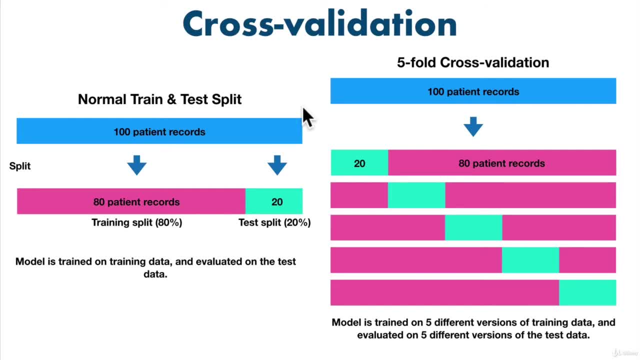 You might do the same to demonstrate what cross-validation is doing, So what we've done before in our normal train and test split. so we've split our data into training. So this could be a state: we started off with a hundred patient records. 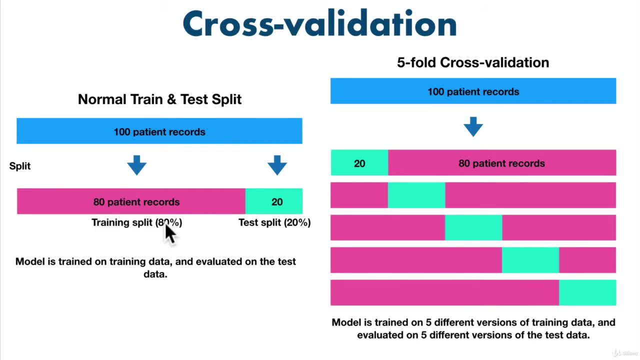 We'd split it into a training split. in our case we've used eighty percent and this would contain X train and Y train, Eighty samples, and I've used the number a hundred. here We've really got more than that, but this is just because the numbers work out visually better here. 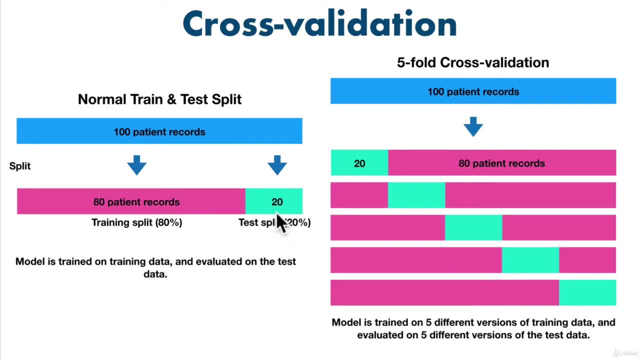 And in our test data set we've got twenty percent of the data which would contain X test and Y train. Now the difference here with cross-validation, and in our case this image here is demonstrating five-fold cross-validation. What you'll probably see cross-validation referred to is K-fold, where K is an arbitrary number. 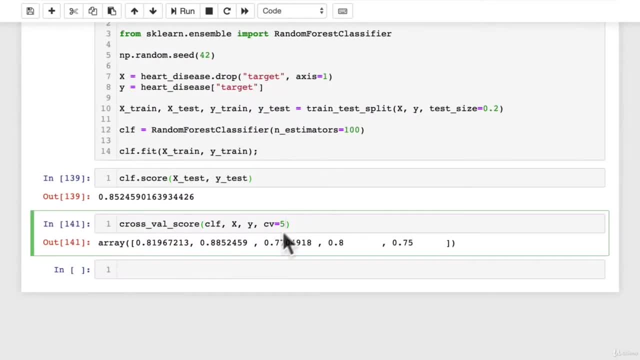 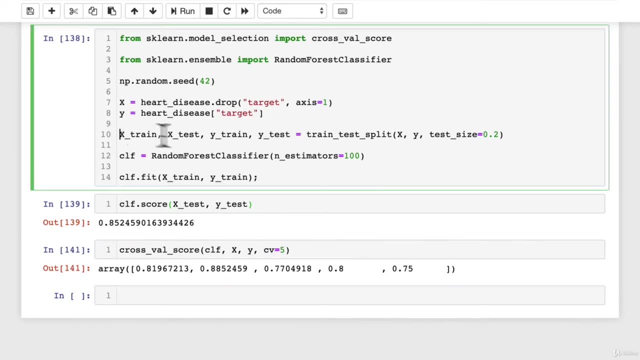 And the reason why we're using five is because, if we come back here, CV equals five there, so that stands for cross-validation, And this is what I'm talking about: splitting our data into training and test, using twenty percent for the test. 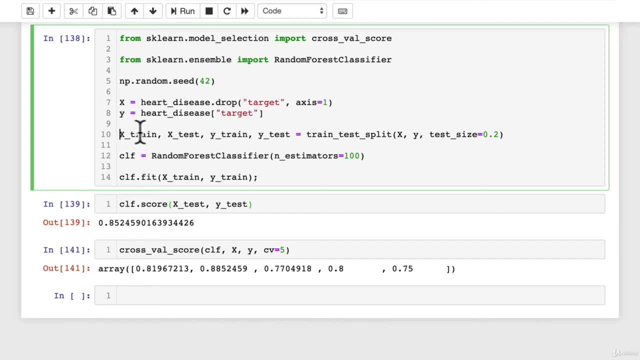 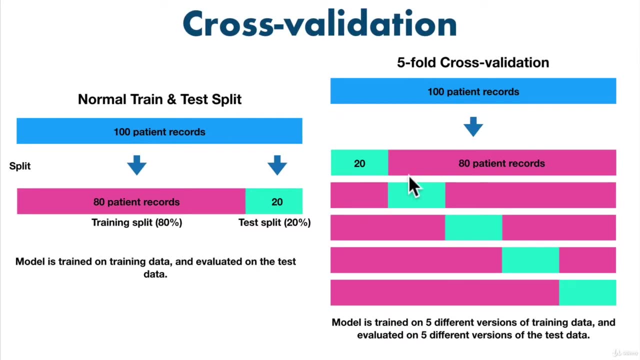 so that means naturally, the other eighty percent goes to the training data, which is where this little split here comes from. Now, what cross-validation does is it does five different splits, So it'll use the first twenty percent. so you see how here this is kind of using the last tail: twenty percent here. 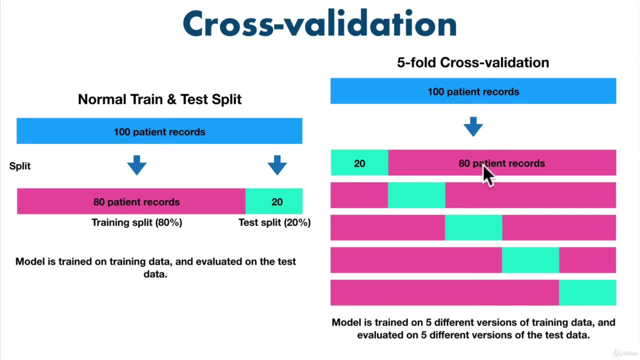 So it'll create a test data set here and a training data set here, Then it'll move over here and use this as the test data set, and then again, and, again, and again. and so what happens is that cross-validation. 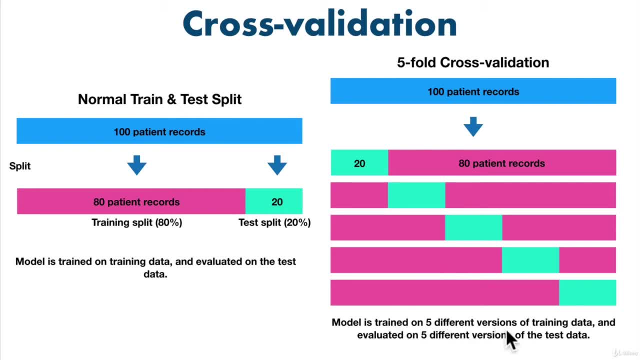 trains five different versions of the model and then it evaluates that those models trained on each training data on five different versions of the test data. So what's the purpose of this? Well, as you can imagine, if we're only training one model, it could be a lucky split. 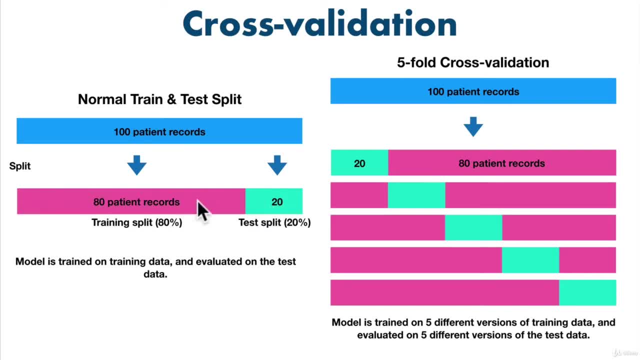 Like, say this: eighty percent of rows say that had Well, as you can imagine, if we're only training one model, it could be a lucky split. Like, say this: eighty percent of rows say that had a whole bunch of information and the model was able to learn really well on these eighty rows, on these eighty patient records. 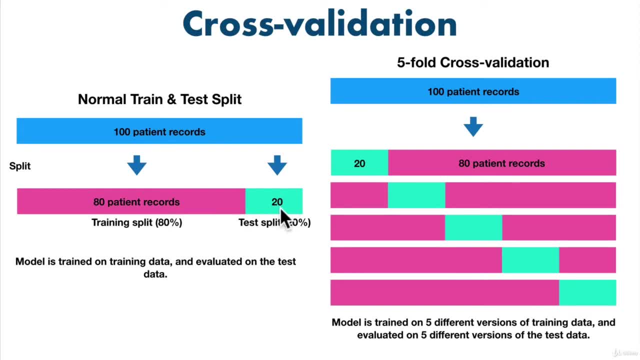 And then it got a really good score on this test set. Is that a true reflection of how our model would understand the data or figure out the patterns in the data? Well, not really. right, Because it's just luck, right, If we're just splitting this randomly? 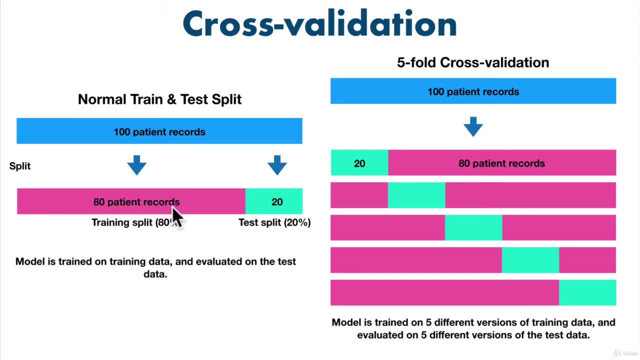 and somehow a bunch of easy patient records have gotten here and the model's figured out certain patterns and it's gone over to here to this test data set and it's got an amazing score. and it's gone over to here to this test data set and it's got an amazing score. 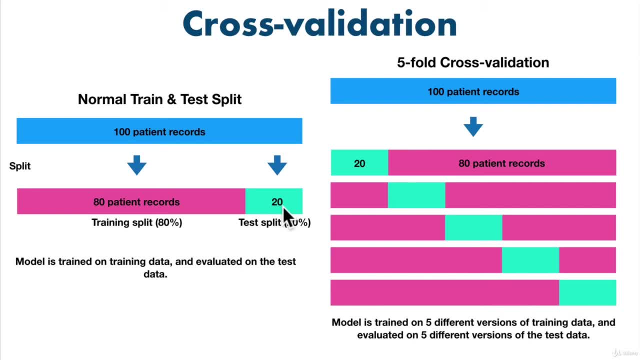 we could be tricking ourselves. we could be fooling ourselves into thinking that our model is far better than what it actually is. So that's where cross-validation comes into play. It aims to provide a solution to not training on all the data. 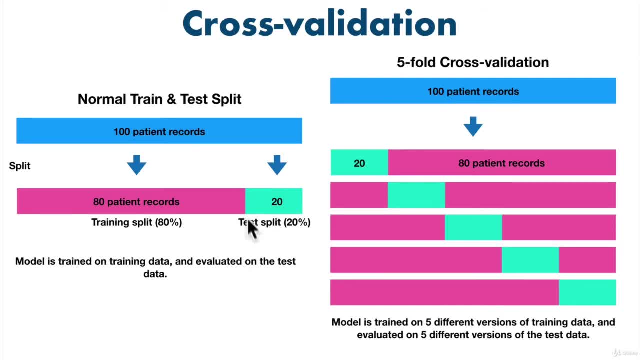 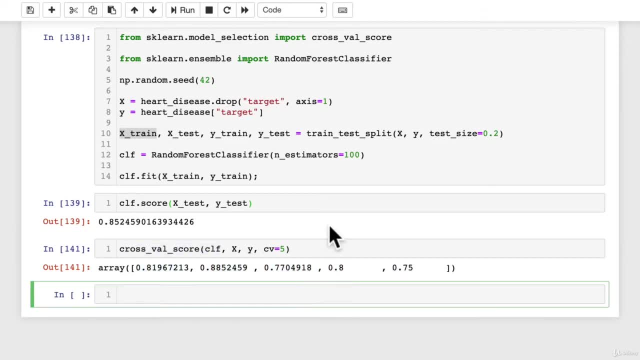 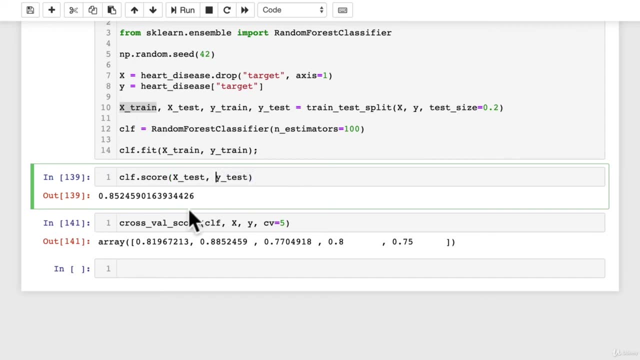 So, no matter what our model is going to be, training on all of the data and evaluated on all of the data, different scores here, ah, so that's starting to make sense. so if we call the score parameter on only our x test data and our y test data, it's going to give back one score. but if we call 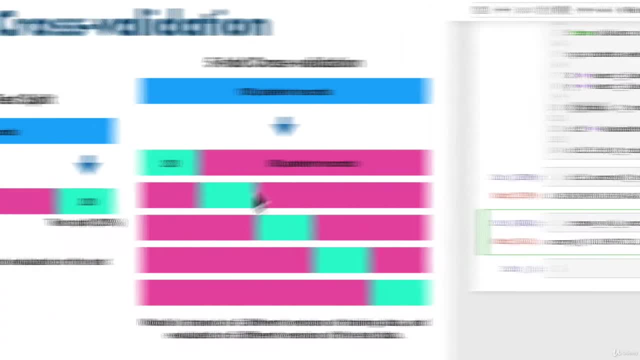 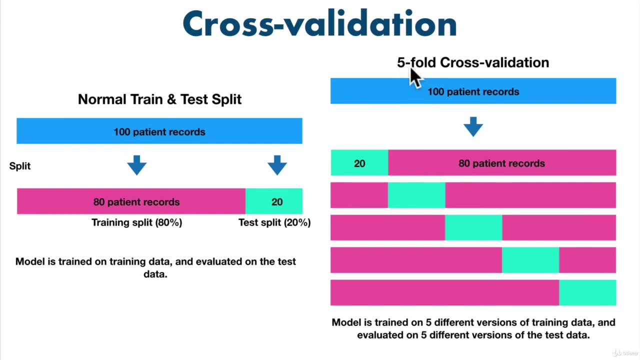 cross vowel score because we refer back to the graphic here. it's going to make five different splits and remember, five fold is just an arbitrary number. you could do tenfold, you could do three fold, you could even do a hundred fold, but five fold is the default of the library and it's usually. 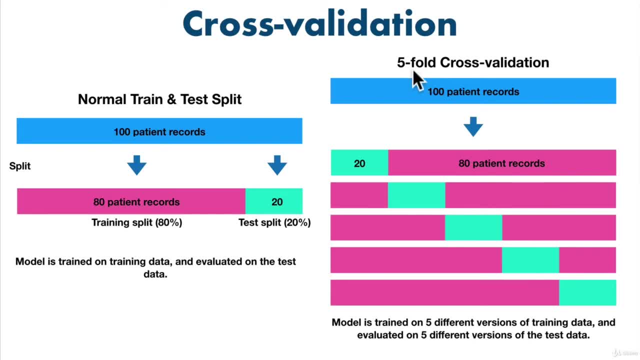 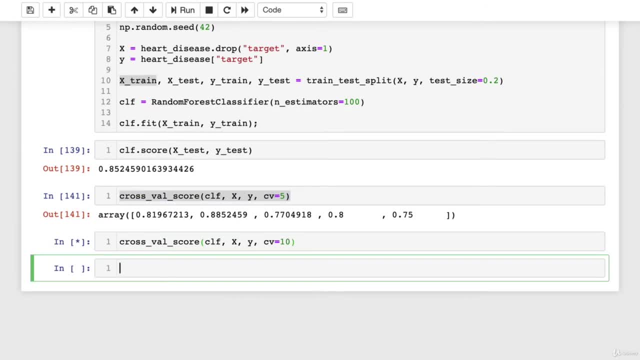 pretty good, depending on the size of your data. so we'll use five fold to demonstrate here, just to prove it to you. we can go in here cross vowel score. we could even do 10. so this means it's just going to make 10 different splits, exactly the same as this, and then return 10. 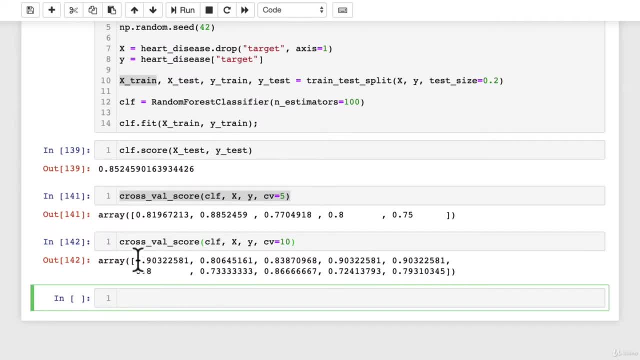 different scores. so you see here this is a great example. on split one it's got a score of 0.9, so that could be 90 percent, which is higher here. but on a later split it's got something much lower- 72- and so what we do here is to figure out a more ideal performance metric or evaluation. 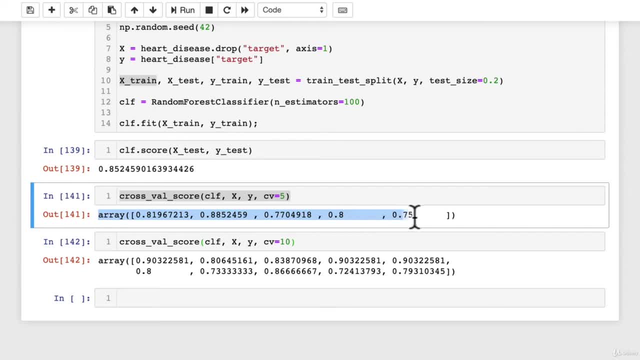 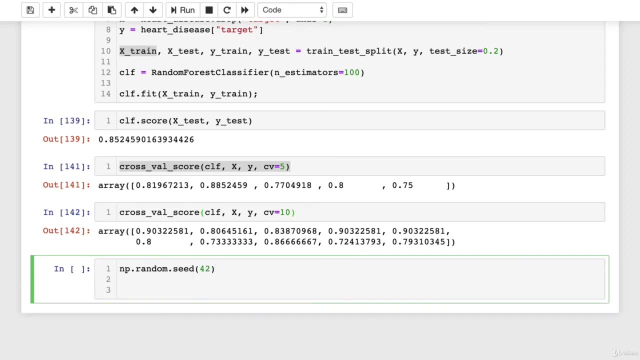 metric for our model is that we can take the average of these five scores. let's see it happen. we'll do it all in one cell, random seed, and what we're going to do is get a single training and test split score. i'm going to make sure. 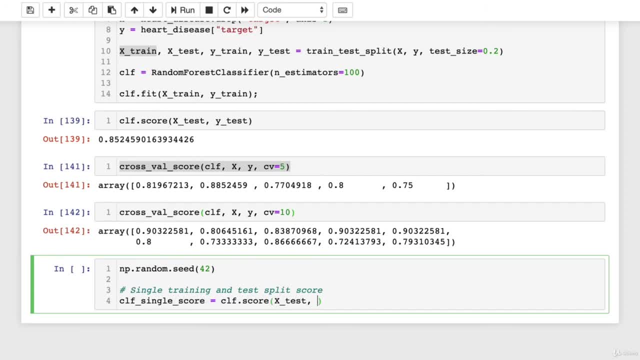 that we get a single score equals clf score. x test. it's going to use the same data here. y test, wonderful. and then we're going to go take mean of five fold cross validation score. clf cross vowel score equals np mean. then we need cross vowel score. 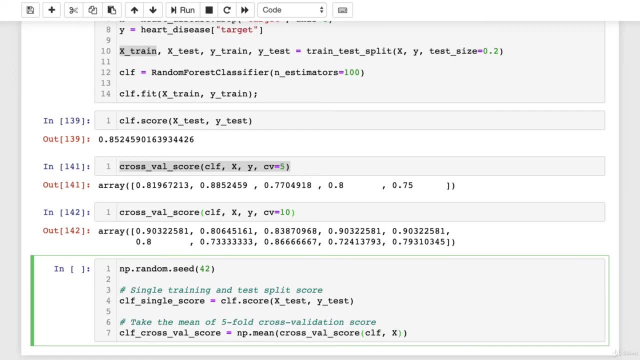 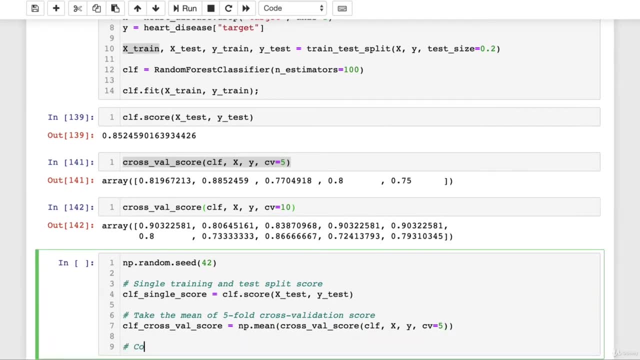 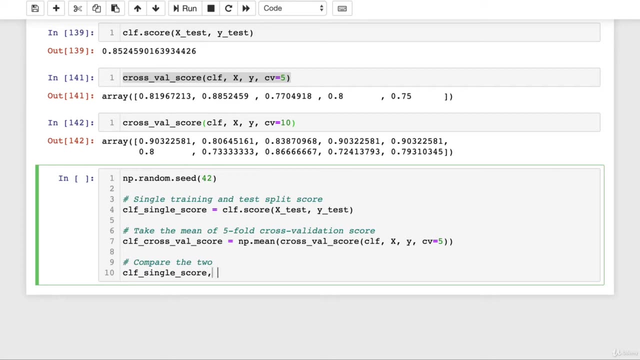 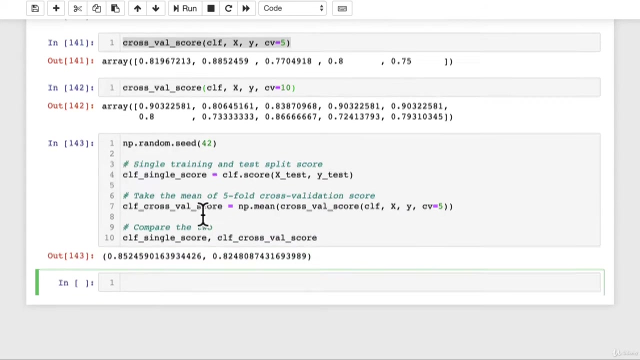 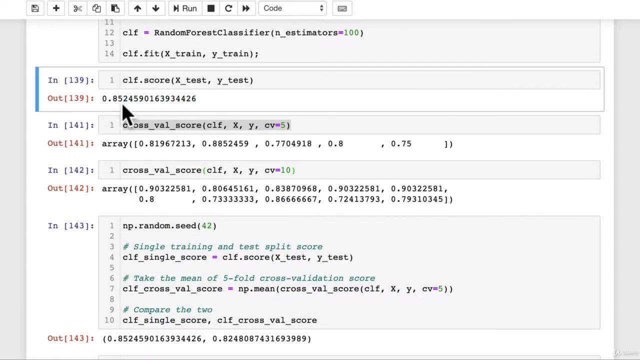 x. oh no, we need to pass it, our classifier x, y, and we'll use cv equals five and then compare the two. so we're going to clf- single score and then clf- cross vowel score. boom. so what do we see here? well, in our case, our original single score, which is now down here just 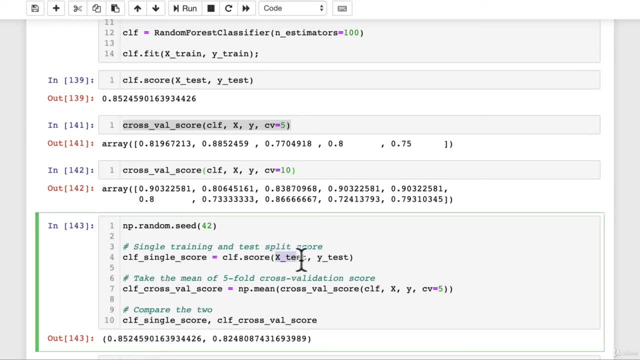 the exact same number because we're using our first cell, y線. we're going to lump it all in double and put that in the second cell now, until we quite completely offset this and move that one number, because we're using a random seed, using the same test data, our single. 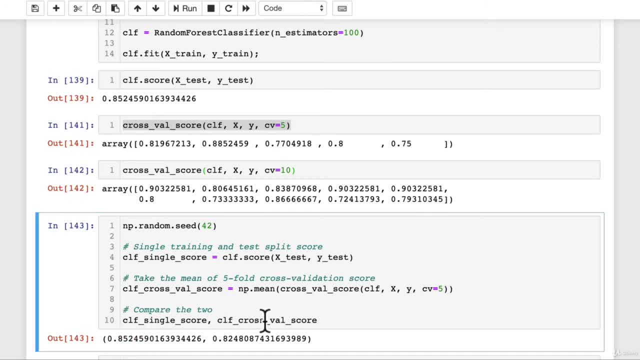 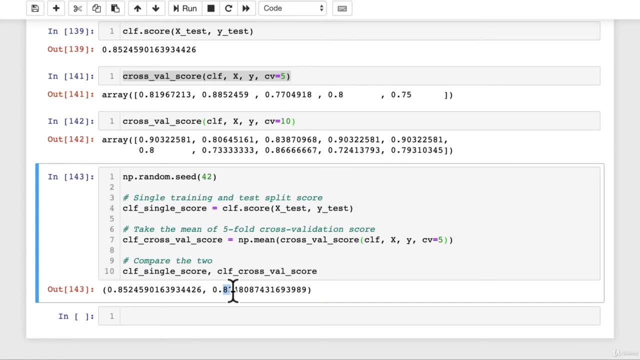 score is 0.85. but when we use cross validation, when we use five splits- because CV equals five- we get a score of 0.82. so it's slightly lower. but in this case, if you are asked to report the accuracy of your model, even though it is, 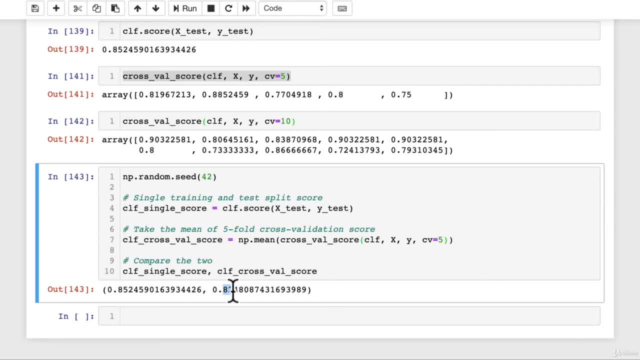 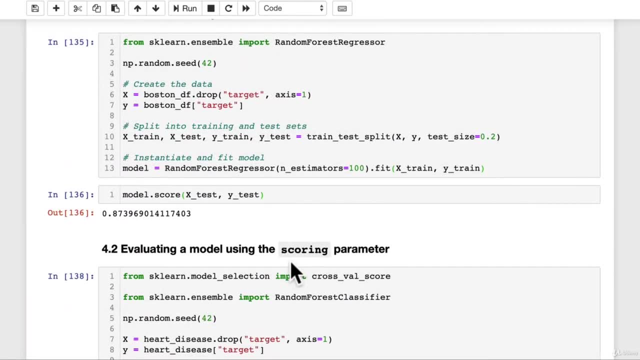 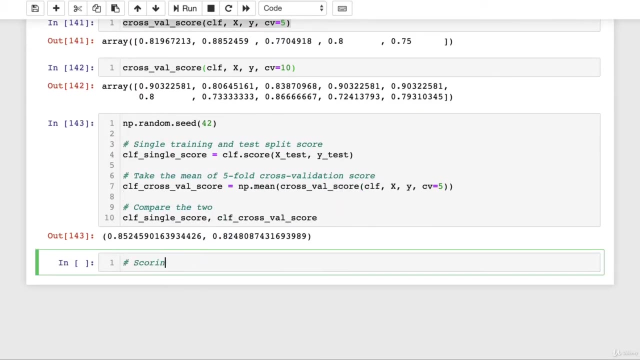 lower. you prefer the cross validation metric over the non cross validation metric. now wait, we haven't even used the scoring parameter at all. well, that's because by default it's set to none. let's have a look. scoring parameter set to none by default. so if we call cross Val score CLF, X, Y, CV, we 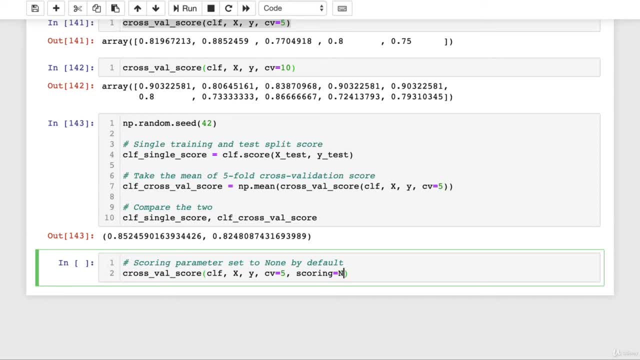 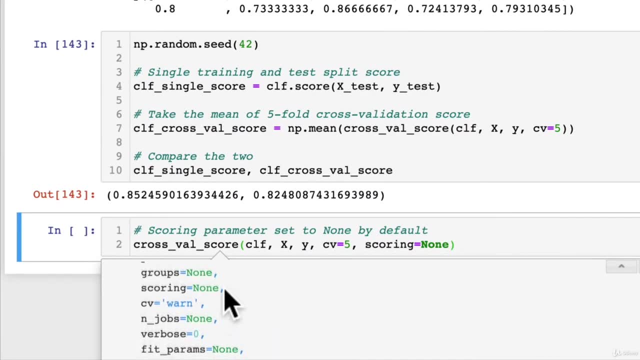 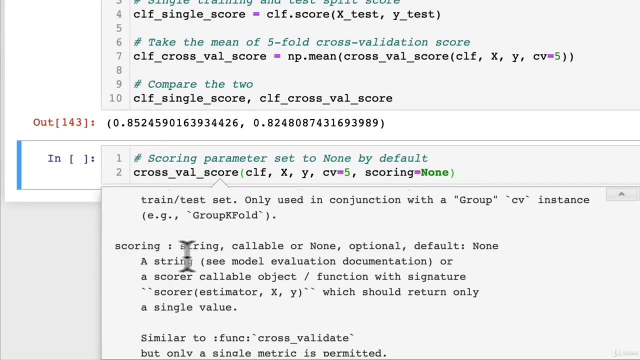 can pass scoring here and it's going to be set to none. so if we do shift tab on this, how do I know this? well, luckily the doc string comes in handy. see, by default it's set to none. so if we keep scrolling down, move our notebook. so scoring string: callable or none. optional default: none. 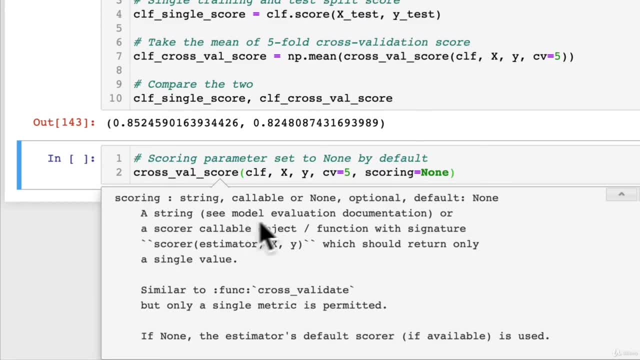 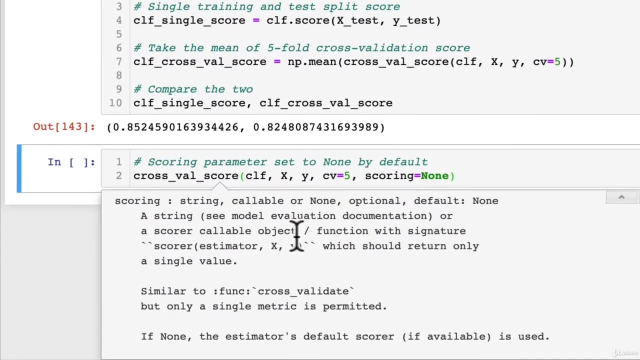 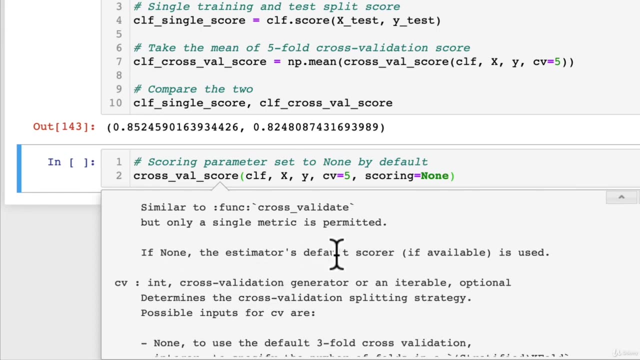 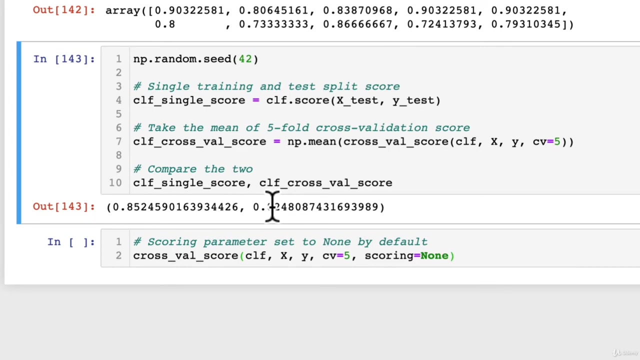 ah, okay, a string: see model evaluation documentation. that's what we've had a look up here. or a score, a callable object slash function with signature scoring. now, this is why we know that this is accuracy, because if the scoring parameter of cross Val score is none, it uses the default scoring parameter of our. 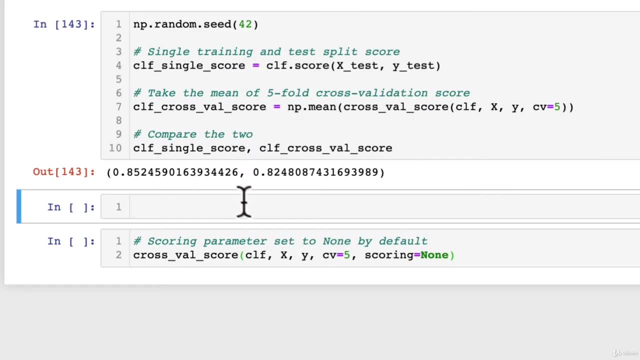 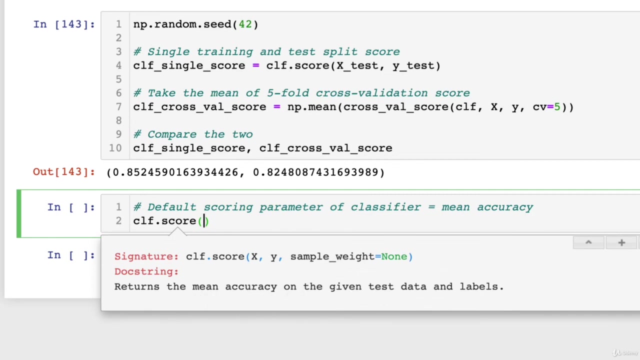 estimator in an. our case, what is it? default scoring parameter of classifier equals mean accuracy. and where did we see that before? we saw that in the last video. when we go CLF dot score and we hit shift tab returns the mean accuracy on the given test data. 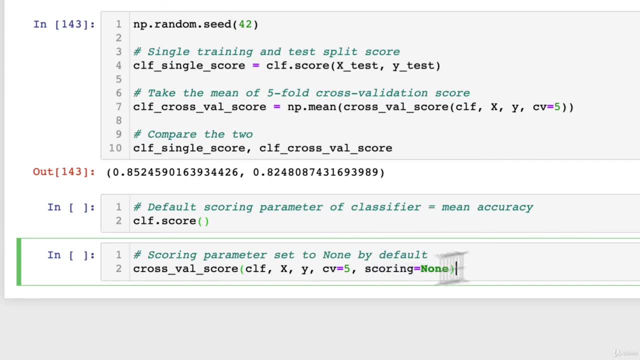 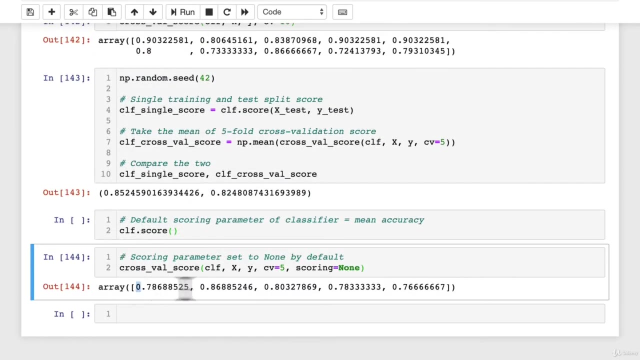 and label. so that means when we have scoring set to none, it's going to use the default evaluation metric for cross validation on our classifier. so if we hit shift and enter, this is going to return the same values or it might be slightly different, right, Because we haven't set up a seed in this cell. 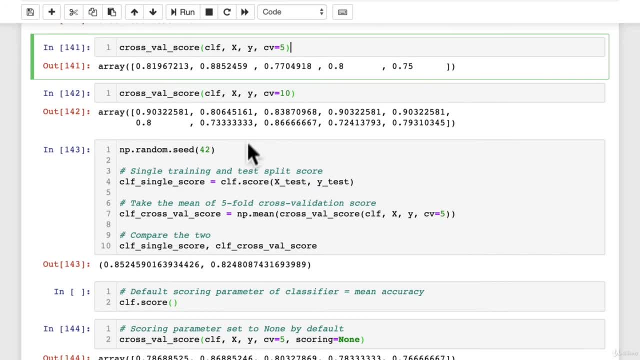 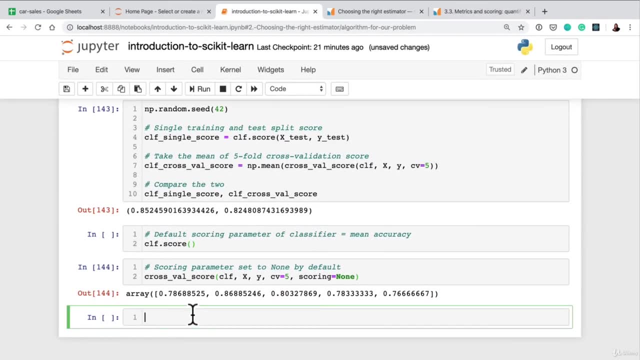 So these values are going to be different to the CrossVal score we see up there. If we'd run it in here, we would have seen similar values. What have we covered here? Well, as you might have guessed, the scoring parameter can be changed, right, So we can, as the doc string says. we 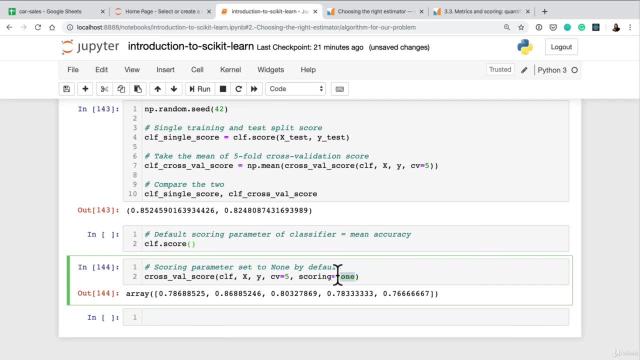 can input our own scoring parameter here. We can change this to something other than none. That is what we're going to start to cover. right, We're going to have a look at in the next few videos some other classification model evaluation metrics that we can use with CrossValidation, And so why? 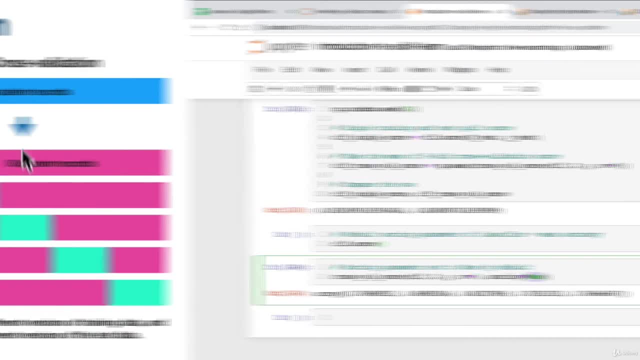 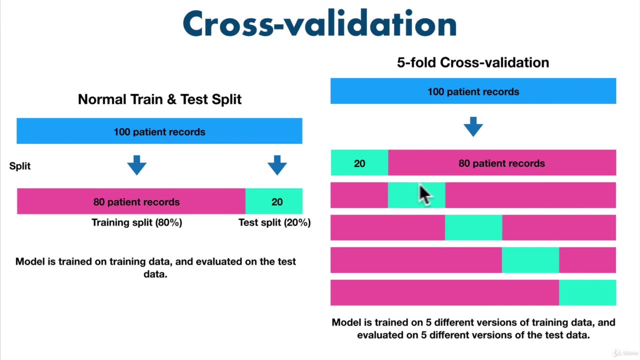 we use CrossValidation Well, as we saw in the picture, CrossValidation aims to solve the problem of not training on all the data, right? So we're creating five models and we end up having a model trained on all of the data and 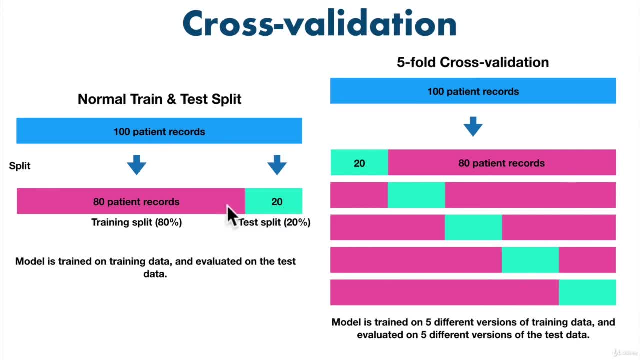 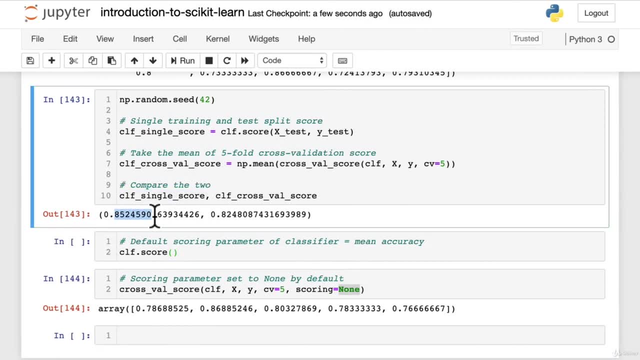 avoiding getting lucky scores. so training on a single split, And we saw that in action, With our single split score here getting a slightly higher score than our CrossValidation score. Whew, That's a lot. Now we've still got a bit more to go. 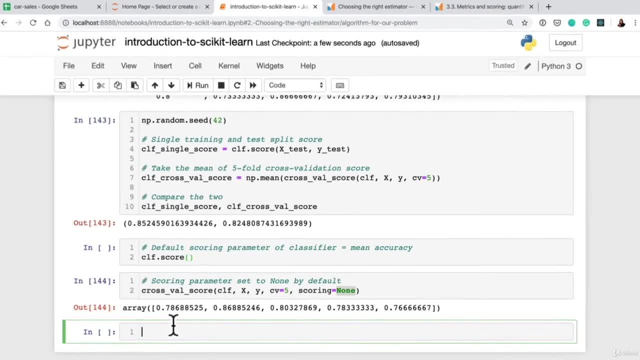 Let's get some in-depth classification metrics happening. I'll see you in the next video. 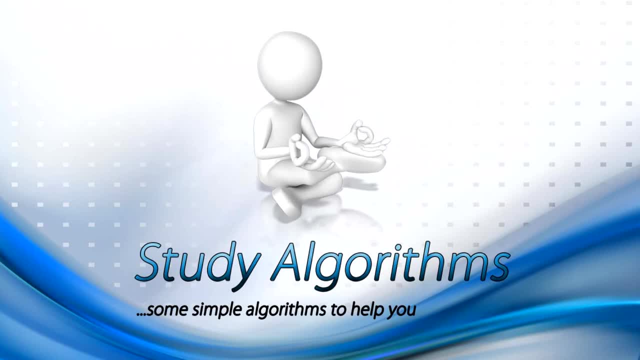 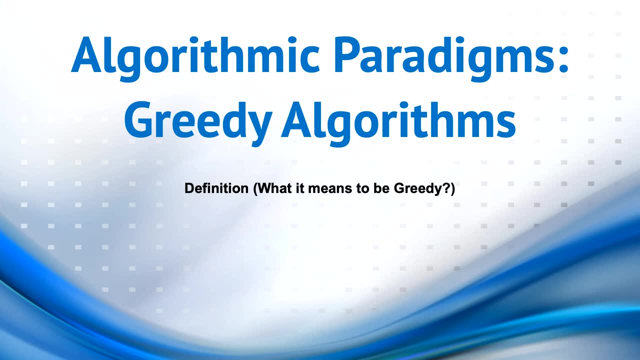 Hello friends, welcome to Study Algorithms, and today we would be looking at Greedy Algorithmic Paradigms. First I would tell you the definition and show you what it means to be greedy. We would then see a real life example and solve it using this paradigm. Going forward, we